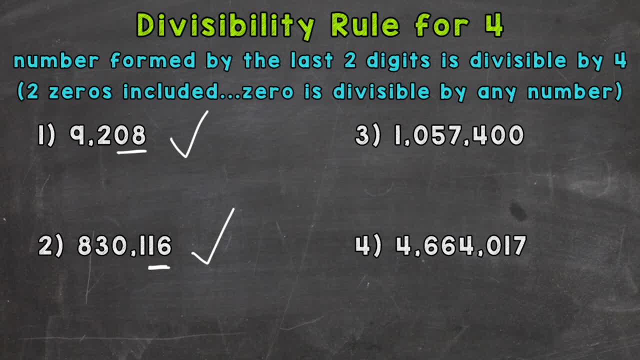 Number 3,, we have 1,057,400.. Last two digits: we have 0 and 0,, which is just 0.. So remember, 0 is divisible by any number, therefore divisible by 4, and that means 1,057,400 is divisible by 4 as well. 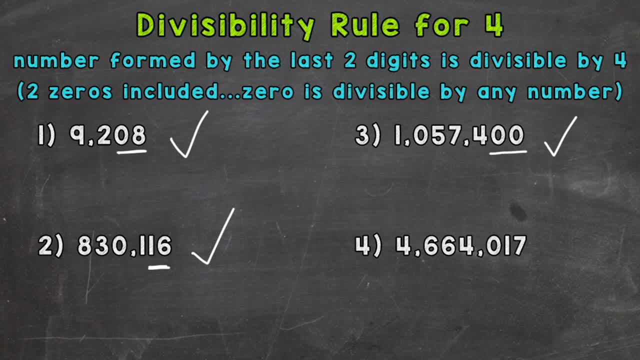 And lastly number 4, we have 4,664,017.. The last two digits, we have 17 here. Now 17 is not divisible by 4, therefore 4,000,000, 664,017 is not divisible by 4 either. so this one is a no. 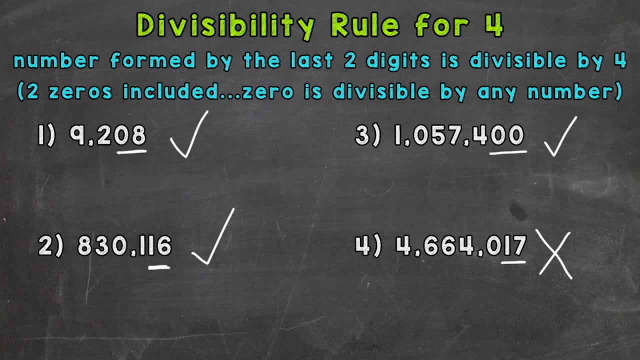 So there you have it. there's the divisibility rule for 4.. I hope that helped. thanks so much for watching, until next time, peace. 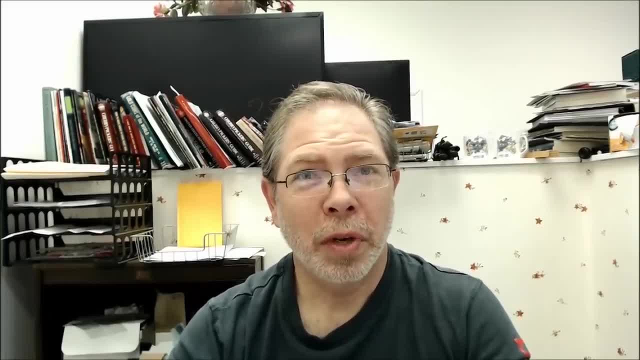 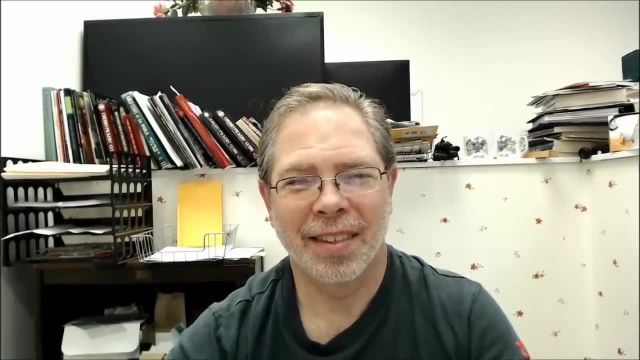 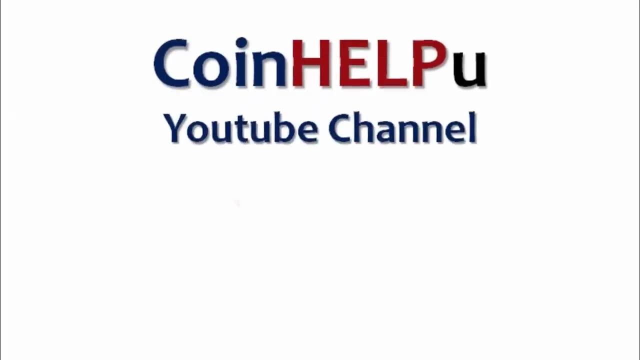 So you don't know anything about coins, but you need to appraise your collection. In this video, we're going to talk about how to do that, so stay tuned. My name is Daniel and you are watching Coin Help U. Thanks for watching my latest video. 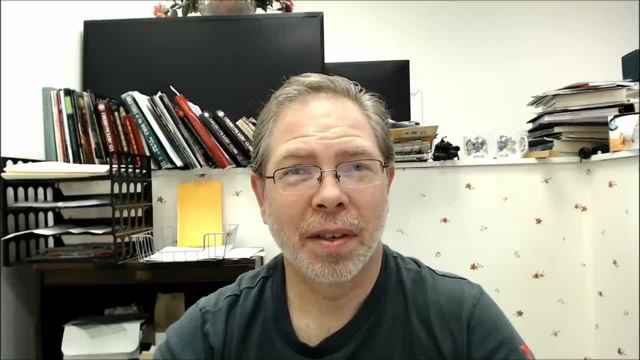 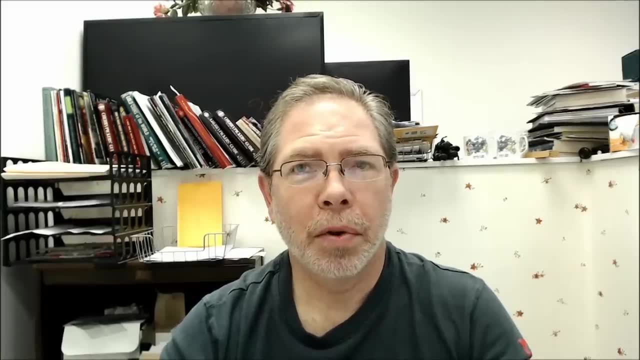 As a long-time coin dealer, I've appraised a lot of collections and I'm going to share with you some of my pros and cons and my taps and tips on how to do that. You know, it doesn't matter whether you have one coin or whether you have a few boxes of coins. Obviously, the larger the 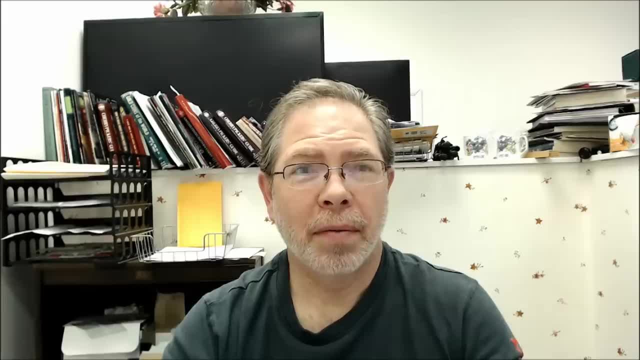 collection, the more difficult this is going to be, but there are a lot of pitfalls and a lot of things that you can fall into whenever you're trying to appraise a collection, and when you don't know about coins, it's time to learn if you're going to appraise it yourself. I know a. 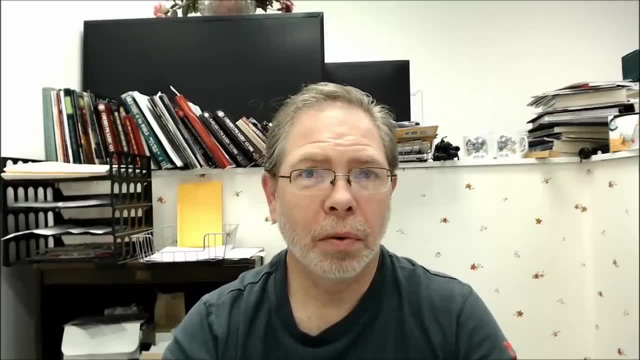 lot of people don't always trust dealers or don't know what dealer to go to. I kind of get that in a way. but you know, it's a lot of people I don't know what dealer to go to. I kind of get that in.